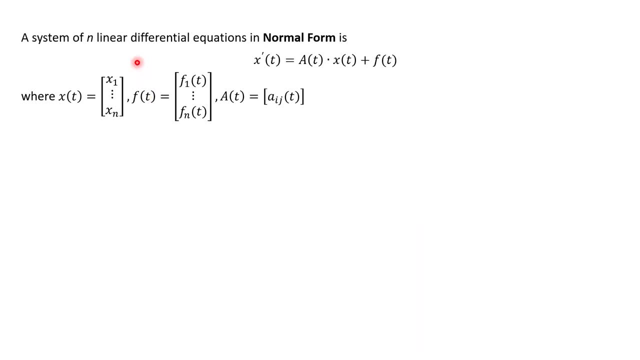 few videos back. So a system of n linear differential equations is called or considered in normal form. if it looks like this: We have x prime, which is a function of t times, or equals a times x plus f of t, And so a, in this case, is going to look like this matrix, and then f you 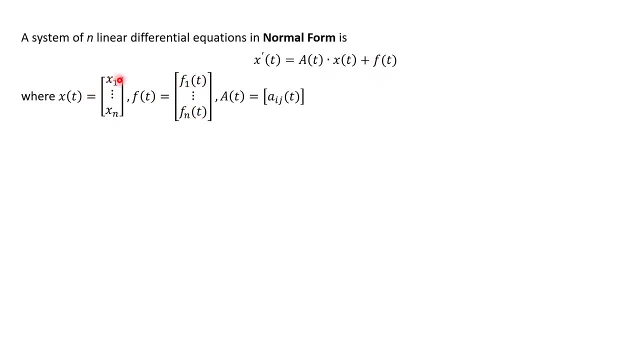 can think of as a vector of functions, x is also a vector of functions of t, And then if you have a homogeneous system of equations, then this is gone over here. This is just plus zero, and if it's a non-homogeneous system, then this is going to equal something. And so recall we talked about 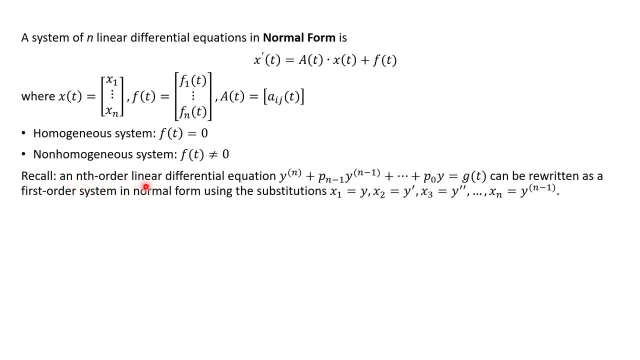 this previously, that you can rewrite an nth order linear differential equation. So in general it would look like this And you can rewrite it as a first order system of linear differential equations in normal form if you start using this substitution. So you can say: well, my function y 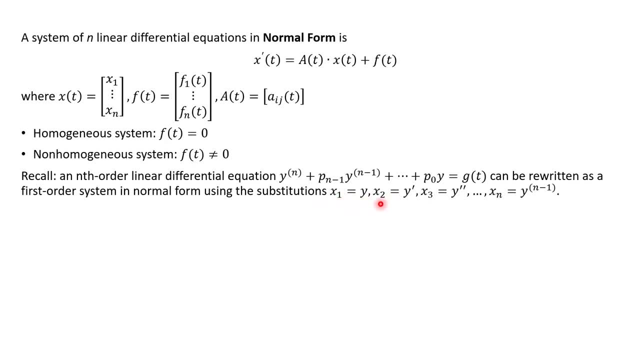 we can call that x sub 1, and then y prime, we can call that x sub 2, y double prime, we can call that x sub 3, and so on. And then we can write this way up to the n minus 1th derivative and we'll call that our variable. or 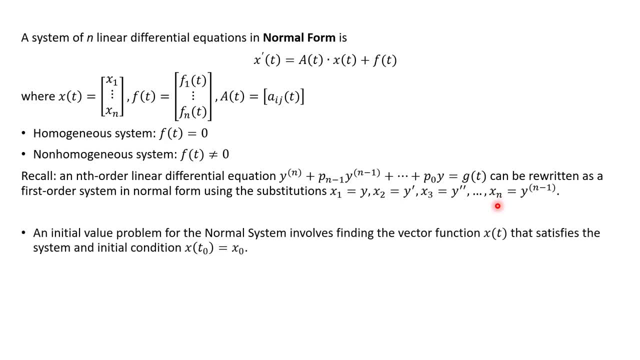 unknown- x sub n, And so you're basically taking an nth order differential equation and writing it as a system of first order differential equations, And so an initial value problem for the normal system just involves finding the vector functions that satisfy the system and the initial conditions. 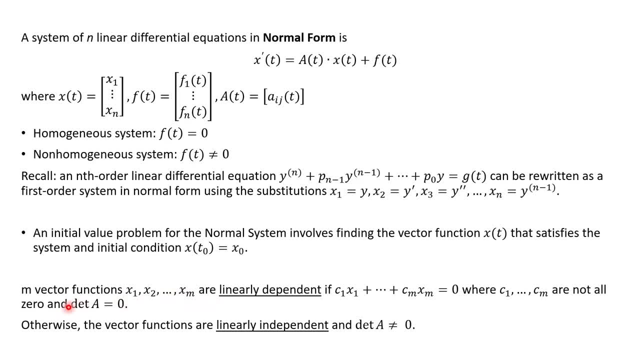 And here's a note about linear independence and dependence. So if we have n vector functions, x sub 1, x sub 2, and so on, if c1 times x1 plus c2 times x2, and so on equals 0, where c1 all the way to cm are not all 0,. 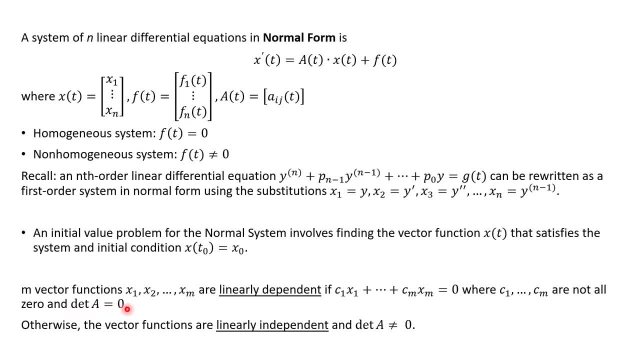 and the determinant of a is 0,, then these vector functions are linearly dependent. So we've talked about linear dependence and independence before, but just letting you know a reminder here: if you can write a linear combination of your vector functions that equals 0,, where not every term is 0, and 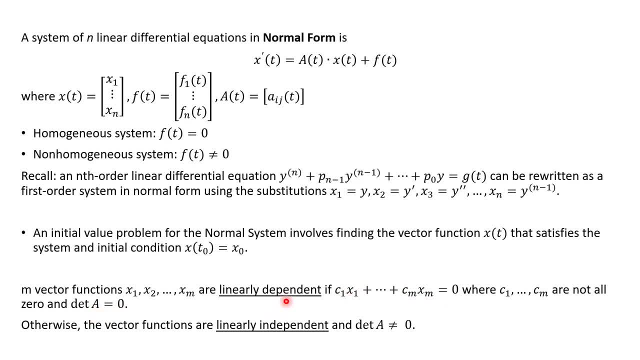 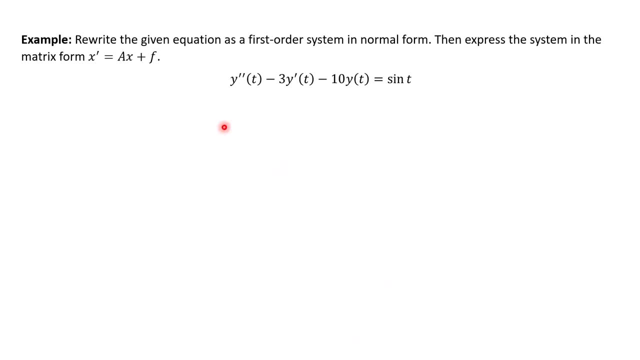 also, the determinant of a is not 0, or is 0,, excuse me, then? linear dependence is the case. Otherwise, the vector functions are linearly independent and the determinant of the matrix a is not 0.. Okay, so let's try out our first example here. We're just going to rewrite our given equation as a first order. 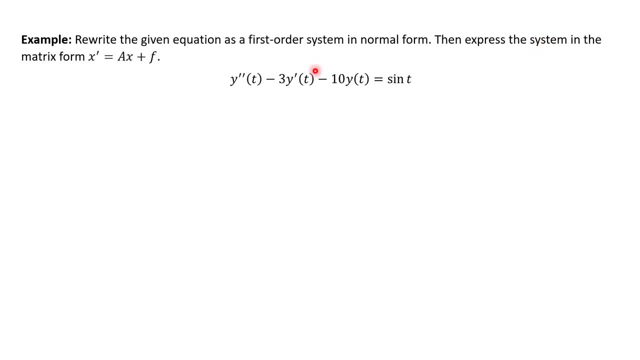 system in normal form and then express the system in matrix form: x prime equals ax plus f. So notice what we're given: a second order differential equation. We want to write it as a system of equations, of first order differential equations. So this is where you 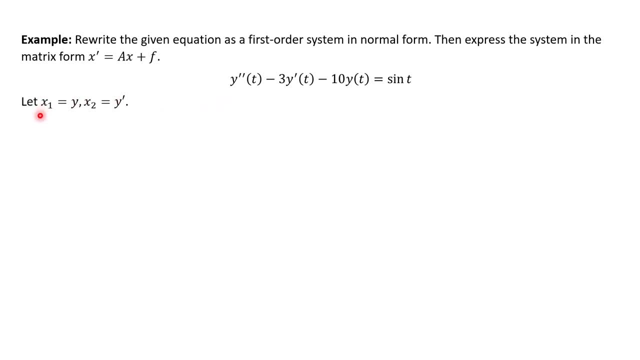 rewrite your variables and you pick some unknowns. So I'm going to say x1 is y and then x2 is y prime, and this will get us up to what we need. We only need to go to the n minus 1 derivative. So, because this is a second order, 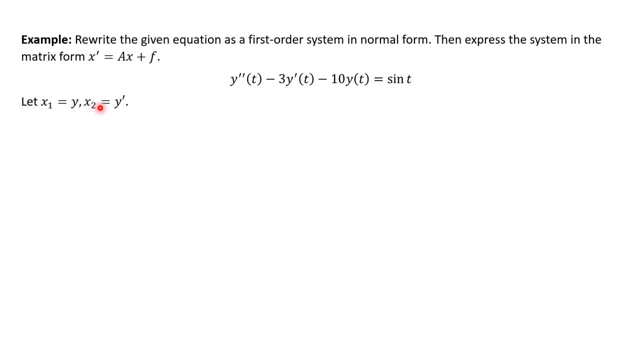 differential equation, we only need to delegate unknowns or variables to up to the first derivative. Quick note, just for example, let's say this was a tenth order differential equation- We would want to define variables up to the ninth derivative. Okay, so now? 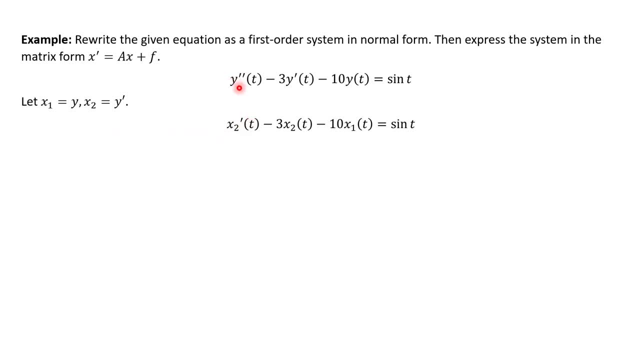 we just replace. We have x2 prime is now y double prime, and then x2 is replacing y prime, then x1 is y. Okay, so now what we want to do is we want to solve for our first derivative. So we have x2 prime and 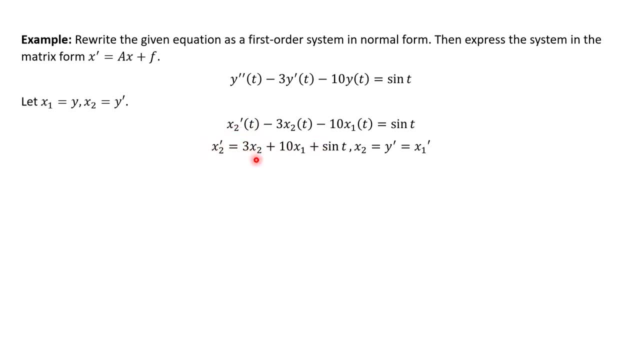 we solved for that. I just took off the t's, but the x's are functions of t's. and then we know from our substitution over here that x2 equals y prime. but we could say that that equals x1 prime. so the first derivative of x1. 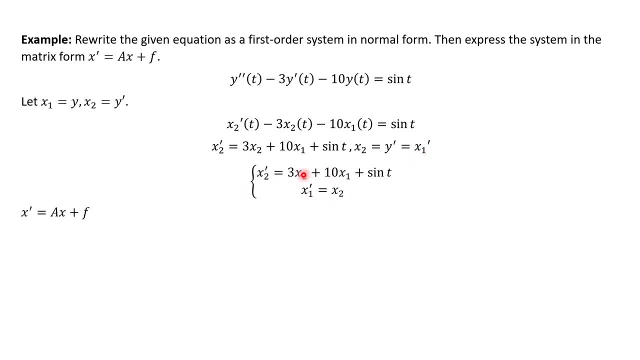 And then that lets us write our system of linear equations, differential equations, as first order equations. So we have x2 prime equals something and then x1 prime equals something. Now let's write it in matrix form. So x prime equals ax plus f, and 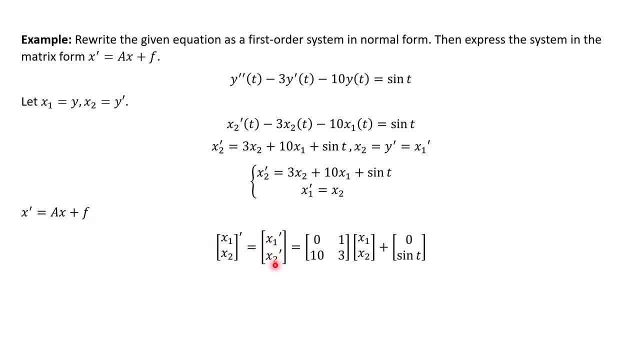 so we just have the vector containing x1 and x2 primes, and then our coefficient matrix- This is a Here's- our vector x and then our terms. over here We do have these terms, this one term that doesn't contain any x's, and 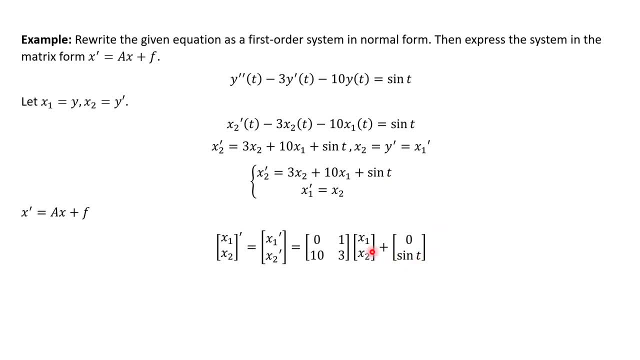 so this is like our non-homogeneous term, and so if you just want to verify real quick, let's just go with x2.. So x2 prime equals 10 times x1 plus 3 times x2 plus sine of t, which is this equation, right here? 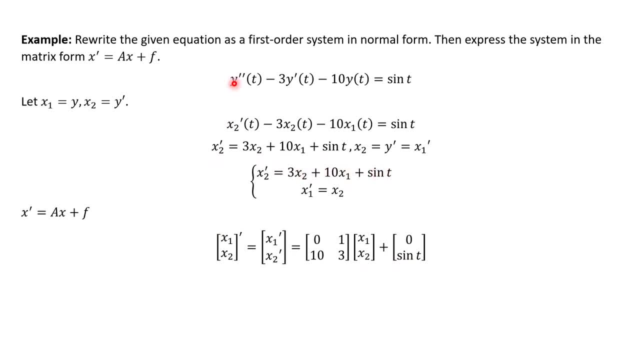 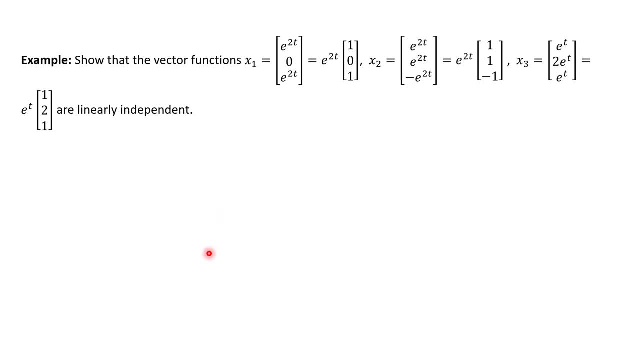 All right. so that's us rewriting our second order differential equation as a system of first order equations And then putting it in our matrix form. Now we're going to be doing some examples with showing linear independence, and so let's show that the vector functions x1,, x2, and x3 are. 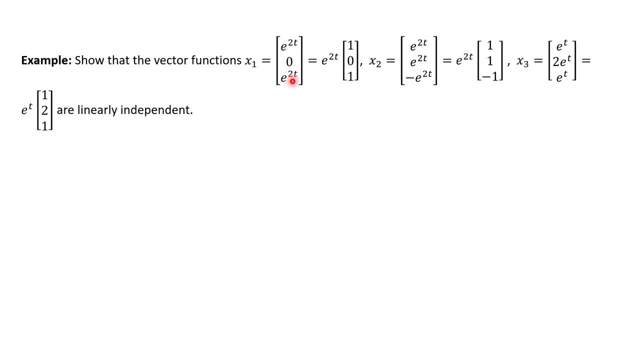 linearly independent. So we have these three vectors given to us and then notice what I did: I just factored out a common factor in each one. So x1, I factored out e to the 2t, x2, same thing, And then x3, we just factor out e. 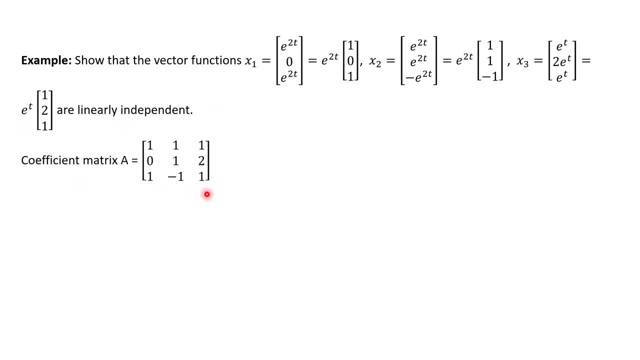 e to the t. Okay, so we have our coefficient matrix that we can form using the coefficients on these vector functions. So notice column 1, 1, 0, 1 comes from x1, the coefficients on e to the 2t, and so on for x2 and x3. 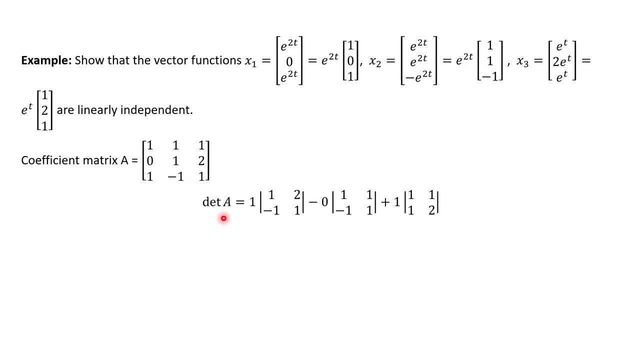 And then we want to verify what the determinant is. So we have the determinant of this coefficient matrix and do your cofactor expansion down any row or column and we end up with some number other than 0, which is good. So then we could say that since the determinant of a is not 0, the vector functions are linearly independent. 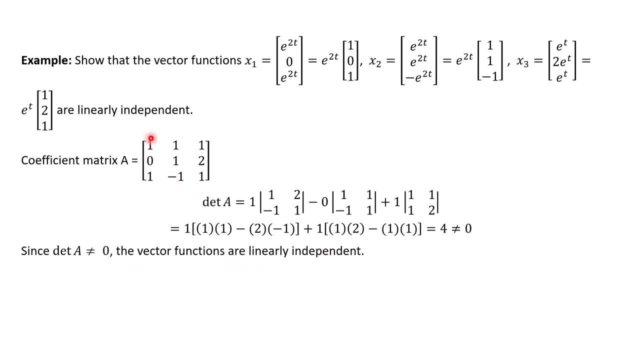 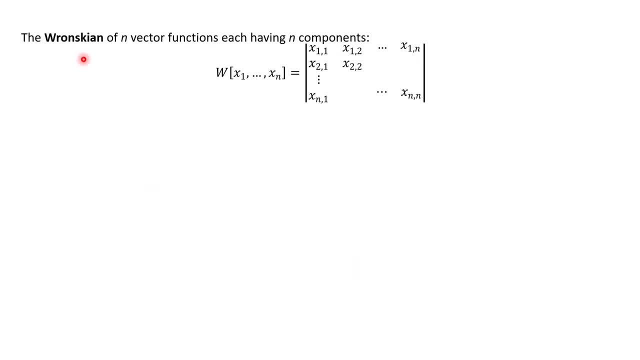 Okay, so just real quick, I did my cofactor expansion down column 1.. All right, now let's review a little bit. We've talked about the Wronskian before, but we're going to use it again here, and it just has a slightly different notation now. 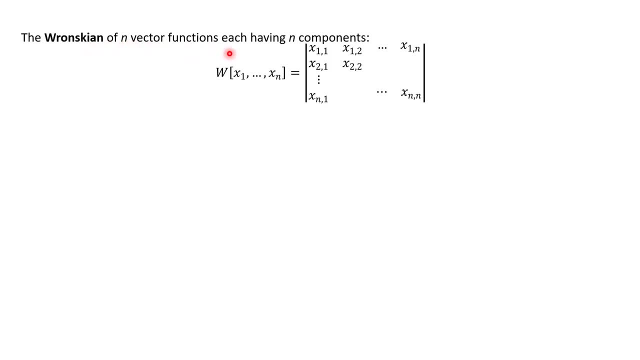 So the Wronskian of n vector functions, each having n components, looks like this. So remember from before: the Wronskian is the determinant of a matrix and so in the past, when we learned it, it was the determinant of the matrix containing the functions and its derivative. 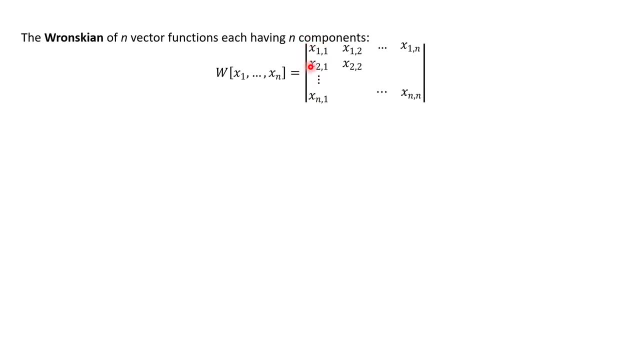 So it's like our function y, then y prime, y double prime, and so on. And so, remember, we were replacing with our substitutions: Our x1 is y, our x2 is y prime, and so on. So that's why the notation has changed. from what we learned, 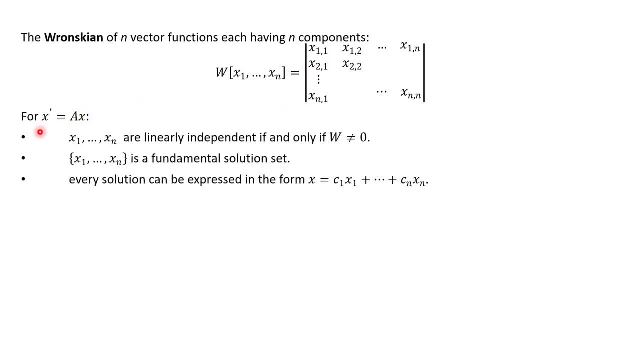 This is what we've seen in the past, And so for our equation x prime equals ax, the following three things are true: Our vector functions x1,, x2, and so on are linearly independent if, and only if, the Wronskian is not 0.. So if, and only if, this determinant 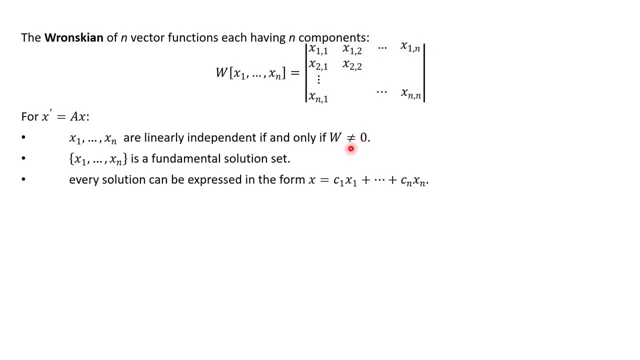 made up of these vector functions is not 0.. And then the set of vectors is considered a fundamental solution set. And then every solution to this equation here can be expressed in the form: x equals a linear combination of x1 all the way to xn. 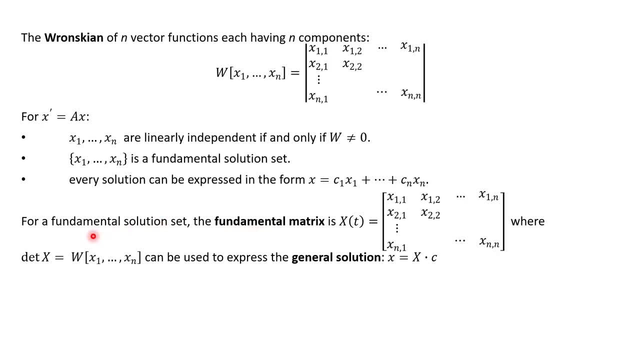 Alright, and so now a definition for us for a fundamental solution set, which is this set here, The fundamental matrix corresponding to that solution set is just the matrix X, capital X. that equals the matrix that's determinant is the Wronskian. So what I want you to notice. it's very subtle. The difference here is that these are vertical lines. 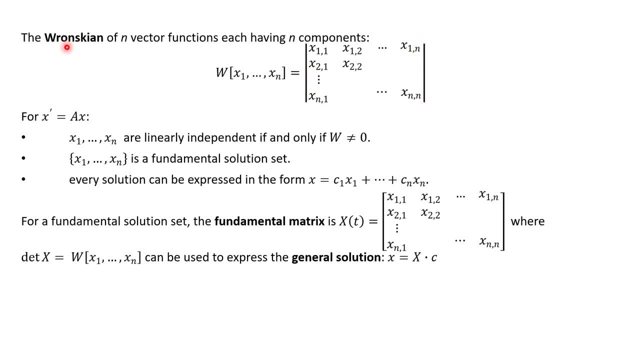 letting you know this is the determinant, and the Wronskian is always a determinant, And over here it's brackets because this is a matrix. Okay, so that's the only difference. The fundamental matrix, the determinant of it, is this Wronskian. 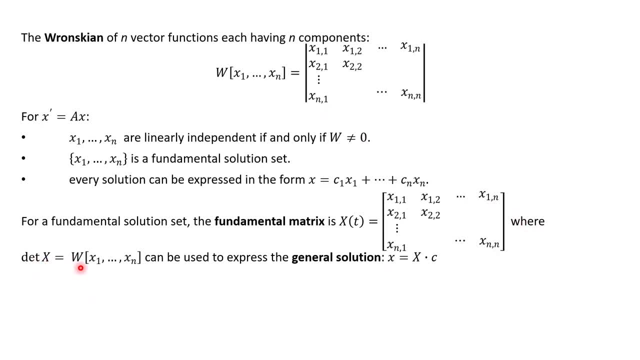 And this is where the determinant of X- exactly what I was just saying- is the Wronskian, And this can be used to express the general solution: x little x equals big X times C. So basically, we're saying that for this. 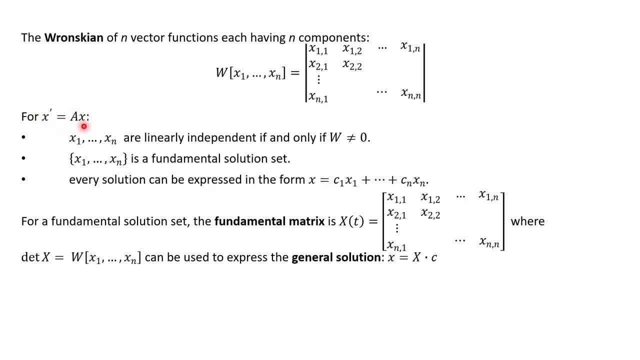 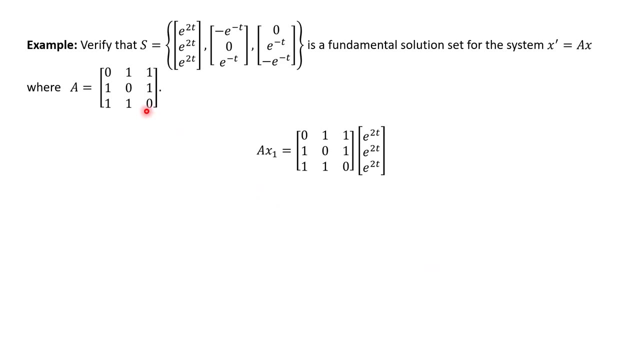 equation right here: X prime equals A times X. the general solution is X and you can write it as this matrix: X times C, which is just some arbitrary constant vector. Alright, so let's work out this example. We are going to verify that this solution set is a fundamental solution set. 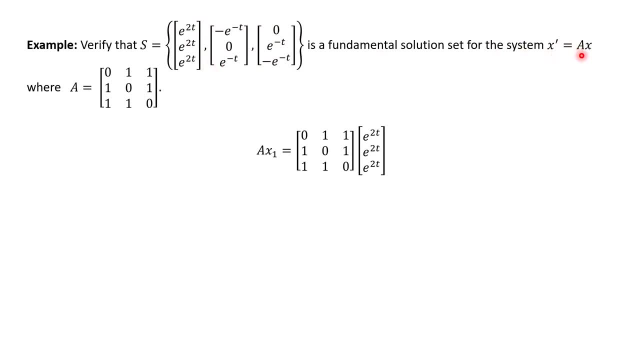 To this system, X prime equals AX, where this is A. Okay, so real quick, notice what you're given. You are given a solution set and we're just verifying that. it is in fact a fundamental solution set to this system of linear first order differential equations and A is given to us. 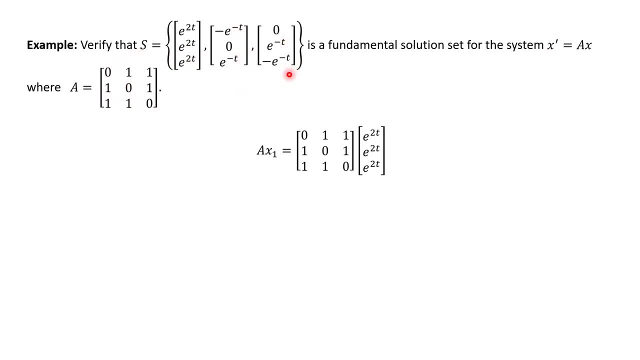 Okay, so this set has three vectors in it. So what we want to do is we want to verify for each one- we're going to call this X1, X2, X3, that each one satisfies this equation. So, starting with X1.. We're just going to multiply matrix A. 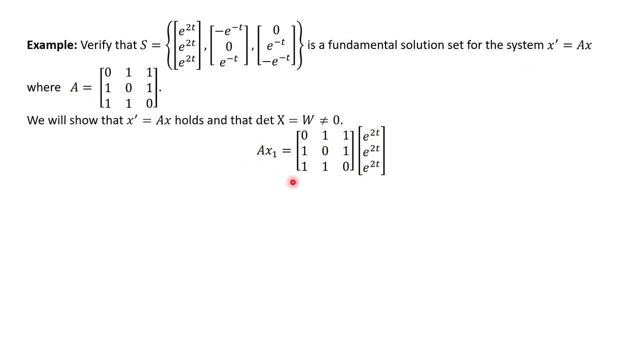 times vector X1, and see what we get. Okay, we want to also show that the determinant of X, which is the Wronskian, is not zero. So it is part of our work here as well. So A times X1, if we just multiply: 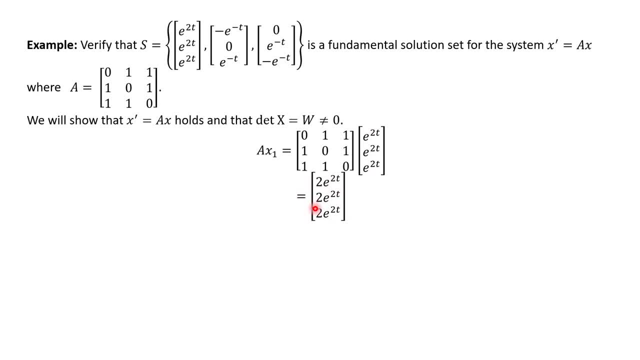 row 1 times column 1, and so on. we're going to get this vector and we want this to equal the other side of the equal sign, so it should equal x prime. So if we differentiate vector x1, we should get this result. if this is in fact the 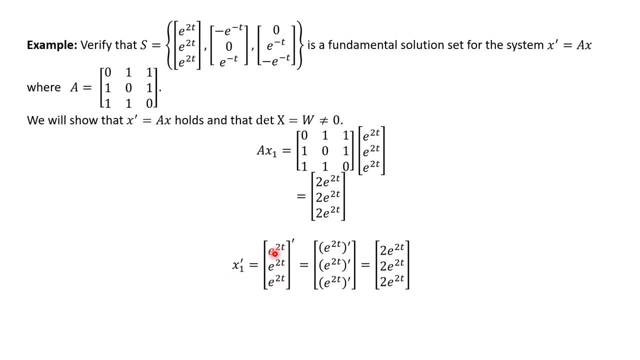 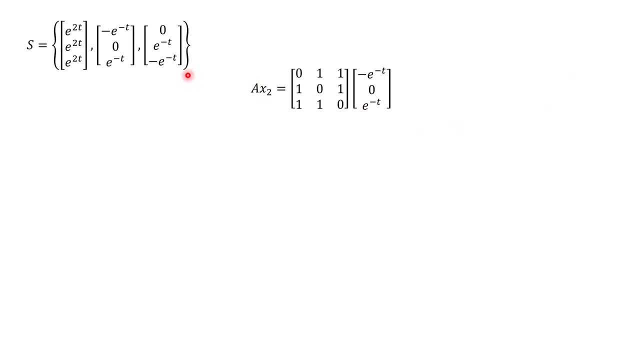 solution, And it is So just differentiate each entry in x1, and it's exactly a times x1.. So this first vector in our solution set does satisfy this equation. So let's do this two more times, So a times x2, multiplying matrix a times vector x2, and here's our result. And then verifying: 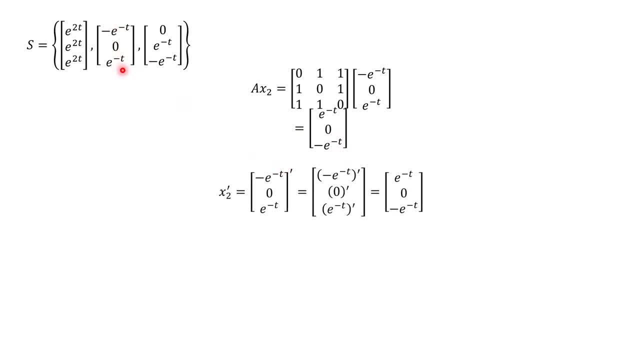 that if we differentiate x2, do we get the same thing. Take the derivative of each entry. and yes, these are equal. So x2 prime equals a times x2, which satisfies our equation One more time doing this with x3. So a times vector x3, that equals this vector here. 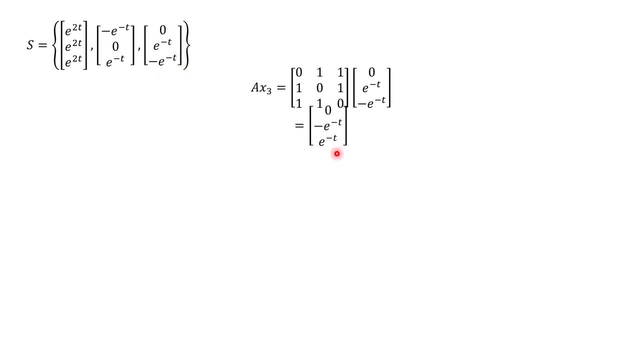 and now we want to verify that if we differentiate x3, we get the same result. And if we differentiate each entry, yes, these are equal. So each of the vectors in our solution set satisfy the equation x prime equals a times x. But we do want to show one more thing. We want 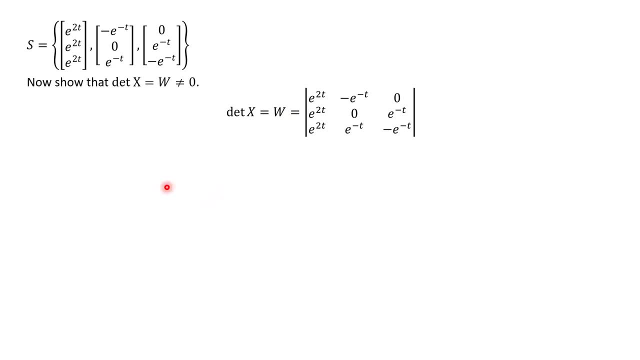 to show that the Wronskian is not zero. Okay, so we're going to compute this determinant And to pick any row or column, I went ahead and just did cofactor expansion across row one and simplified, and we got something other than zero. 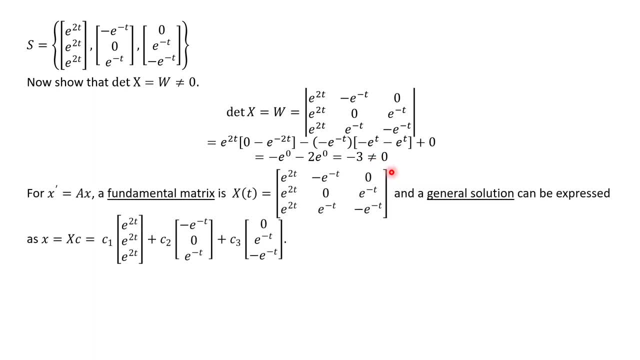 This is negative three, and so that's good. And so we showed that this determinant, this Wronskian, was not zero. So for x, prime equals ax. a fundamental matrix is the matrix capital X, which is a matrix whose columns are the vectors that make up our fundamental solution set. 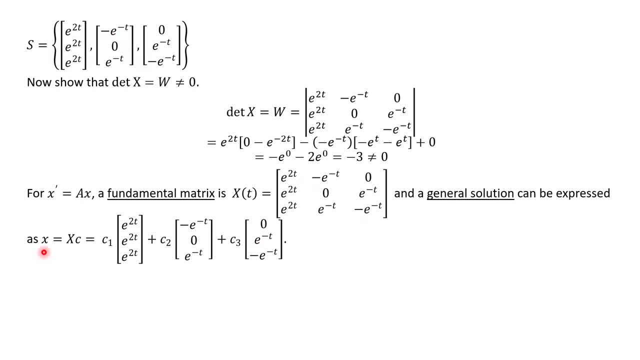 And then a general solution can be expressed in this way: Little x equals capital X times C, which is capital X, which is our vectors that make up the columns of X times these arbitrary constants C1, C2, and C3. 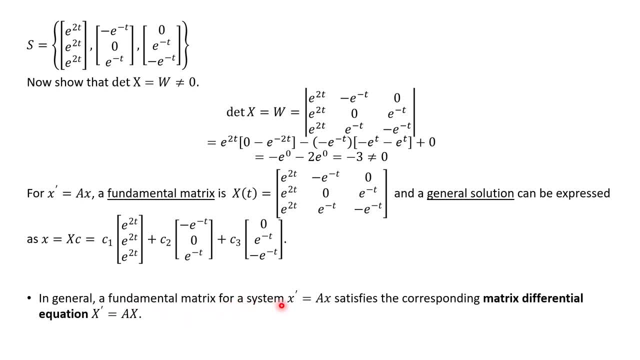 All right, and so, in general, a fundamental matrix for a system, x prime equals ax satisfies the corresponding matrix, differential equation, And so everything. this is fairly the same from what we've been doing, just we're calling it different things and the format might look a little different, And so we're calling this instead of just a regular. 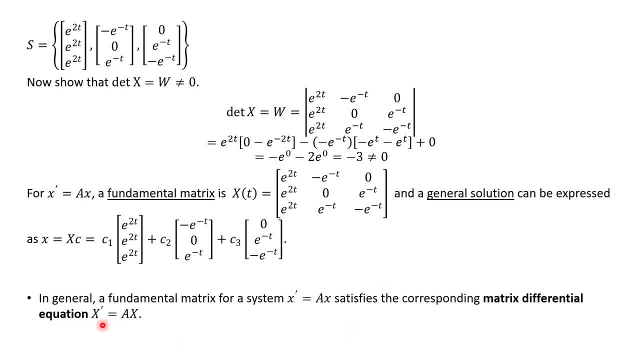 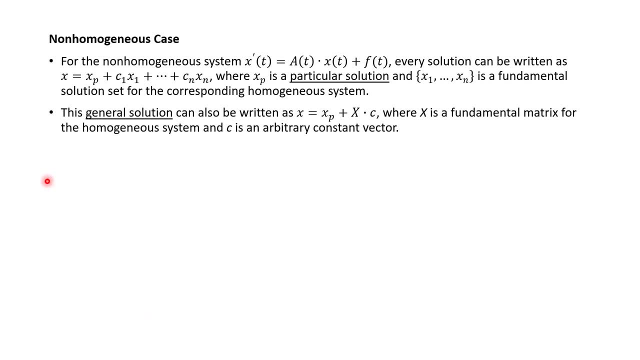 differential equation. we're calling it a matrix differential equation because of the way we've formatted our equation. All right, now the last thing to talk about here is the non-homogeneous case, and then steps for solving. So first for the non-homogeneous case, if we have a system, 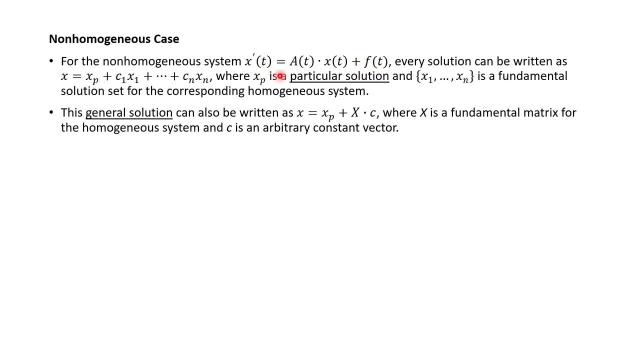 notice what we have over here. this plus f of t. So x prime equals ax or a of t times x of t plus f of t. Every solution can be written in the following format: Notice: the only difference from our homogeneous case is this extra term, which is our extra function: x sub p. So this is where x sub p.